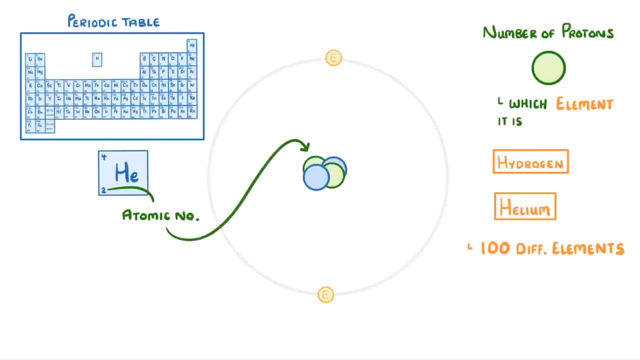 is unique to that element as it represents the number of protons in the atoms of that element, And any atom with that many protons must be that element. So our atom here, which has two protons, must be helium, because helium's atomic number is two. Or if we take carbon, 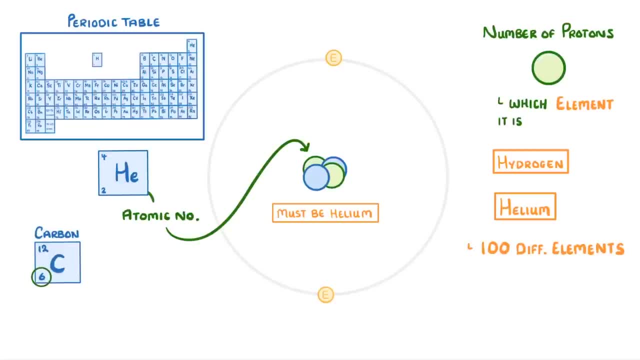 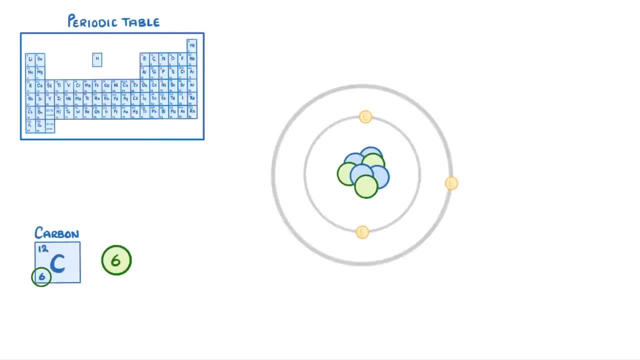 we can see that its atomic number is two. So all carbon atoms have six protons. So if we found an atom with three protons, like this one here, then it couldn't be carbon. We'd have to find the element with an atomic number of three which, if we check the periodic 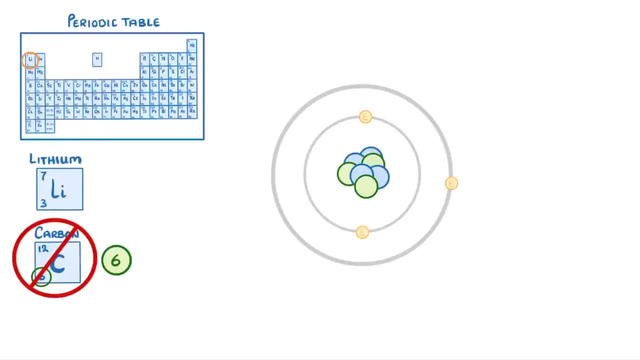 table is lithium. Another feature of nuclear symbols is the one or two letter symbol that represents the element name. So C stands for carbon And Li means lithium. Some symbols, though, are a bit more confusing. For example, sodium is Na And iron is Fe. 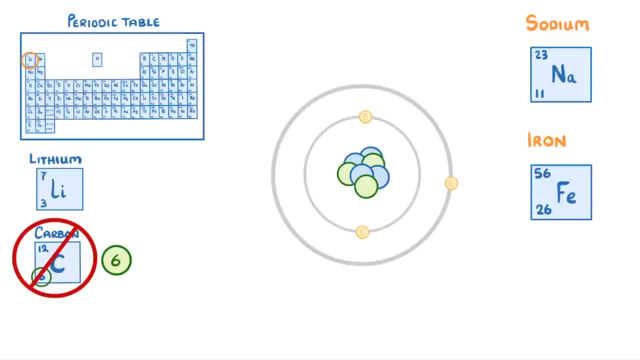 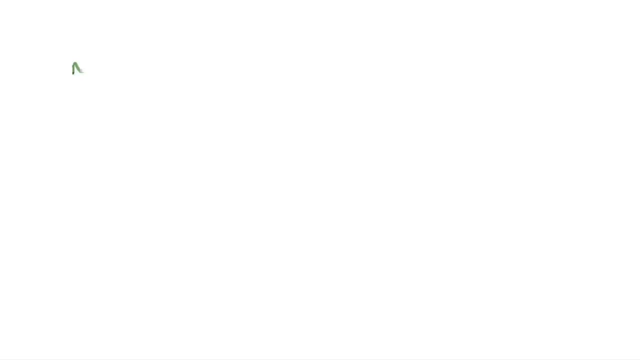 Most periodic tables have both the symbol and the name though, So if you're not sure what a certain symbol is, you can just find it on the periodic table and check. So now that we know that it's the number of protons that determines which element it is, 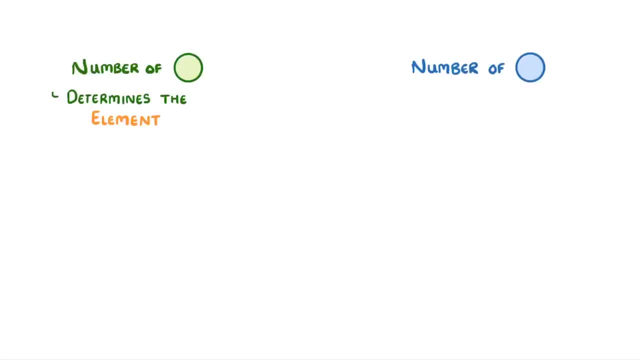 what about the number of neutrons? Well, the number of neutrons can actually vary between the individual atoms of an element. As long as the number of protons remains the same, it's still the same element, And we call these different forms of that element isotopes. 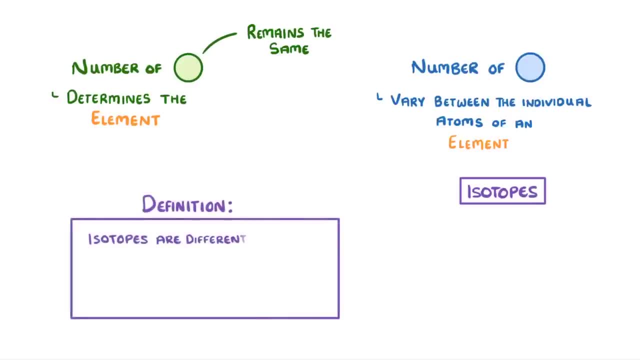 The definition which you need to remember is: isotopes are different forms of the same element that have the same number of protons but a different number of neutrons. Let's take a look at carbon to show you what we mean. The most common form of carbon is so-called carbon-12, which has 6 protons, 6 neutrons. 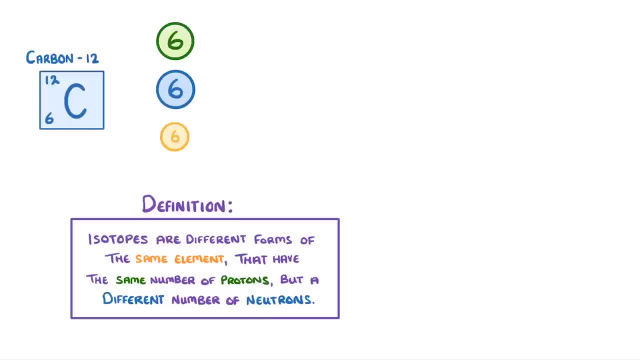 and 6 electrons. A rarer form is the isotope carbon-13, which of course still has 6 protons, because it's carbon, but has 7 neutrons and 6 electrons. This means that it has a mass number of 13. 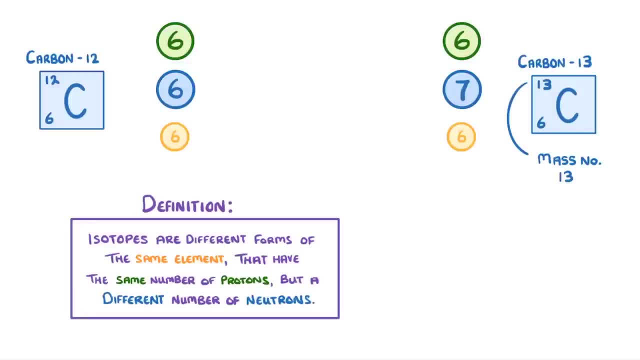 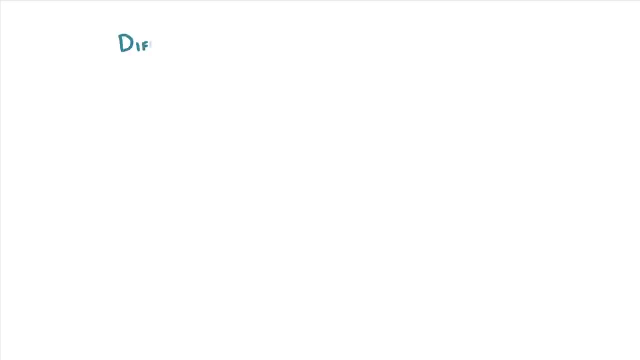 rather than 12, which is why we call it carbon-13.. Because isotopes only vary in the number of neutrons they have. chemically, they all react in basically the same way. Now, because they all have different numbers of neutrons, the different isotopes will have. 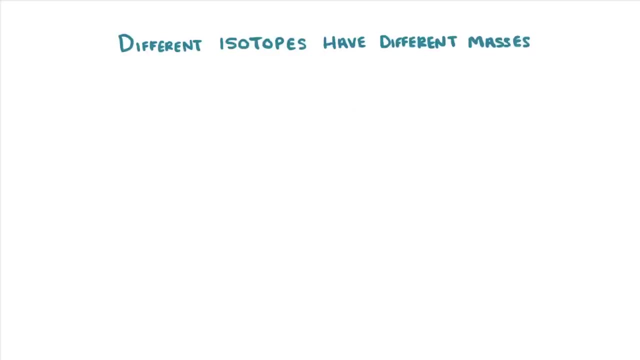 different masses, And one of the things that you need to be able to do is calculate the average mass of all the isotopes that make up a particular element, Which we call the relative atomic mass. Let's take a look at copper as an example. 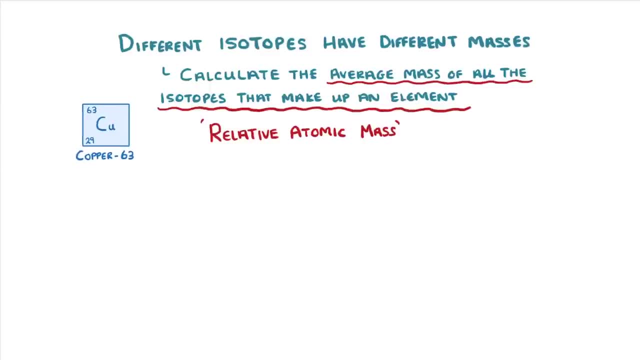 Now copper has two stable isotopes: copper-63,, which has an abundance of 69.2%, and copper-65,, which has an abundance of 30.8%. And when we say abundance all we mean is how common or rare that isotope is. 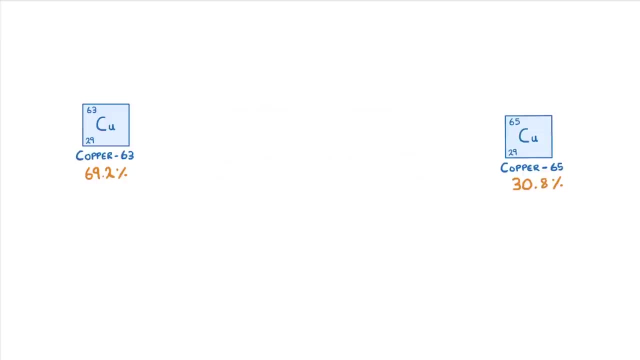 So if you were to pick up a handful of copper, Then on average, 69.2% of the atoms in your hand would be the copper-63 isotope And the other 30.8% would be the copper-65 form. 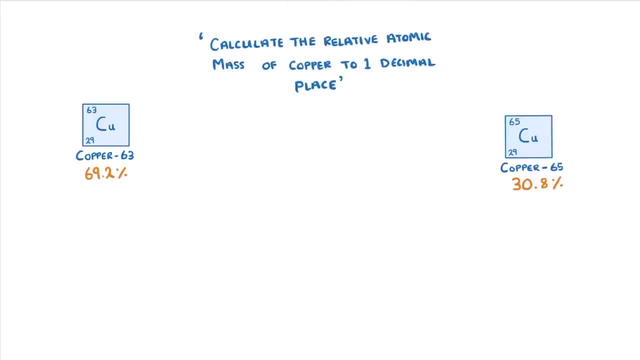 Now in an exam you might get a question like: calculate the relative atomic mass of copper to one decimal place? The equation for relative atomic mass is the sum of isotope abundance times, isotope mass divided by the sum of the abundances of all the isotopes. 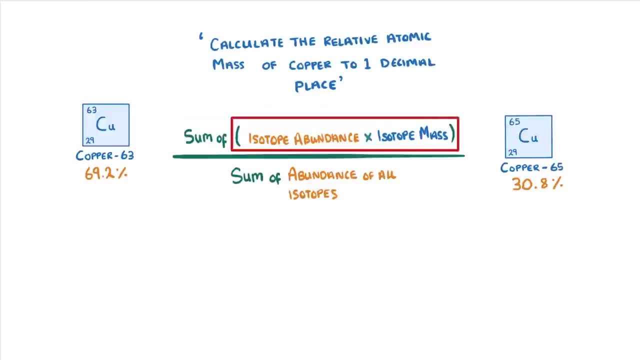 So the first thing we do is multiply each isotope's abundance by its mass. So for the copper-63 isotope, this would be 69.2, which is its abundance times 63, which is its mass. And for copper-65, it would be 30.8 times 65. 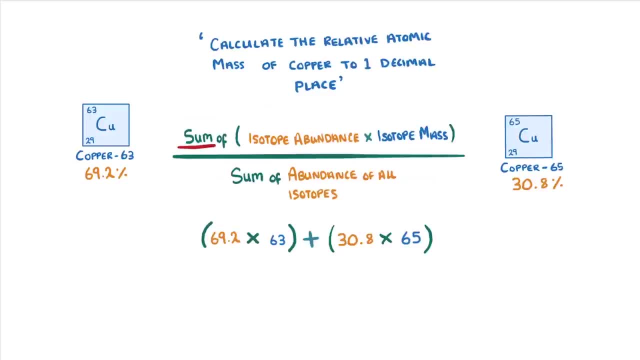 Then we sum these two figures together, Which just means we add them together. Lastly, we divide this by the sum of the abundances of all the isotopes, Which in this case would be 69.2 plus 30.8.. Now you can either put this all straight into your calculator or simplify it down first,